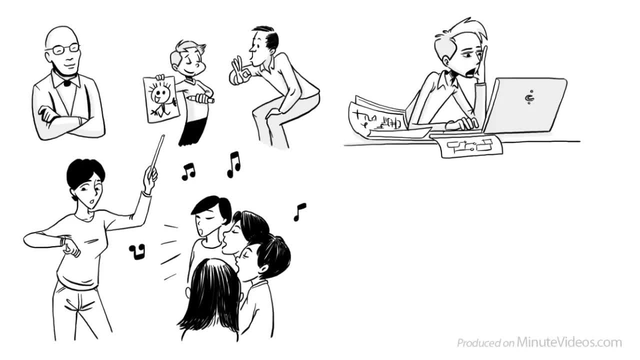 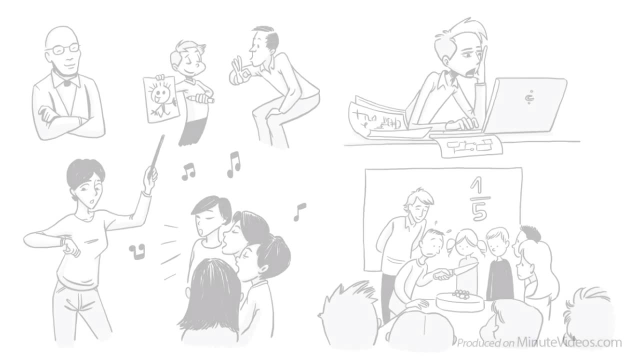 Instead, master instructors have high expectations and maximize the lesson time, But, most importantly, They combine quality instruction with pedagogical content: knowledge. They don't teach a subject, they teach their students how to learn it for themselves. In order to get it right, we have to treat and train teachers like brain surgeons. 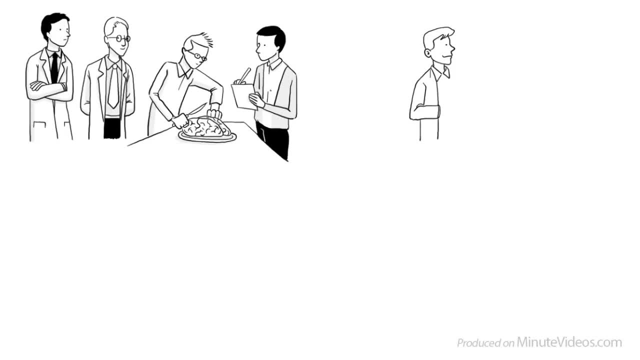 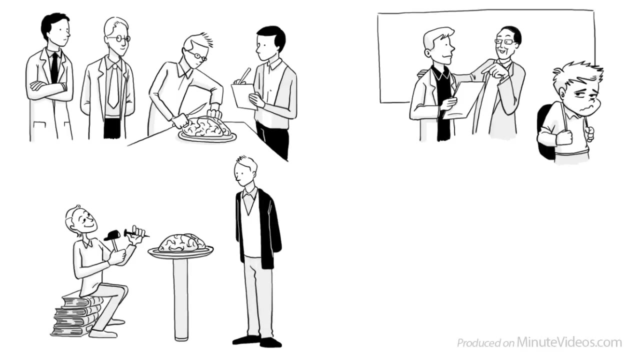 After all, they operate on human brains. Like aspiring doctors, they are best trained in the field where they receive professional feedback when they make mistakes. Effective schools of education therefore train teaching like a craft rather than an abstract science. At Spasato, a graduate school of education known for creating effective teachers, students 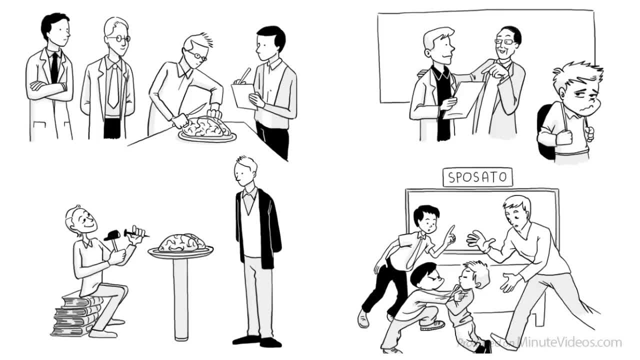 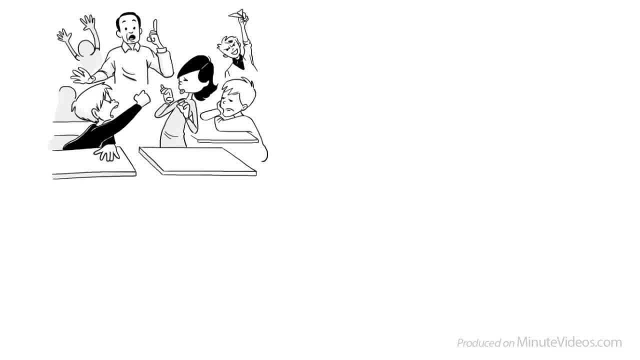 spend a lot of their time tutoring or assisting professionals. Teachers who are already in the classroom need regular professional feedback on the job. A vast study by Roland Fryer from Harvard found that teachers who receive precise instruction together with specific, regular feedback from a lead teacher will improve the most. 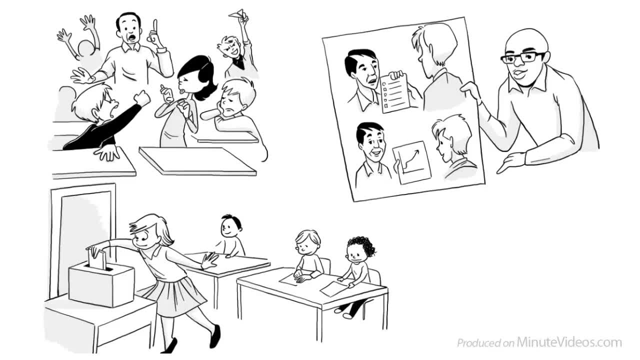 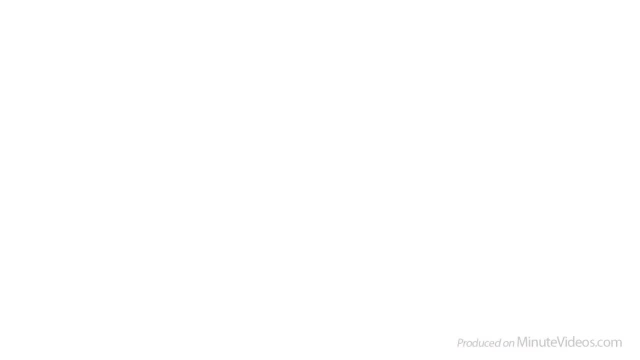 Other good ideas to improve teachers are to ask the students for feedback or to record lessons on video and let the teachers watch themselves. Doug LaMov, founder of Uncommon Schools and author of Teach Like a Champion, identified many methods that great teachers use. 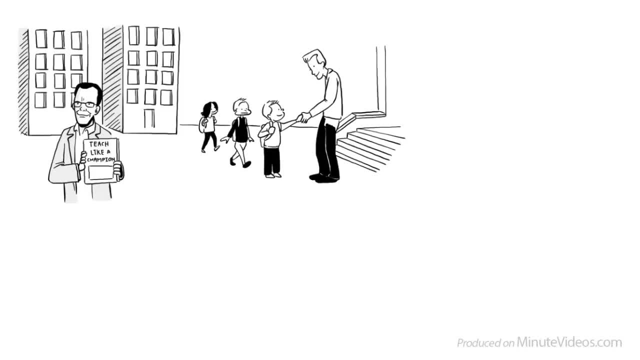 They greet each student at the door so students feel welcomed and accepted. They also teach the students how to learn. Students are taught how to be more creative or how to be more successful. They also teach the students to be more open or to be more objective. 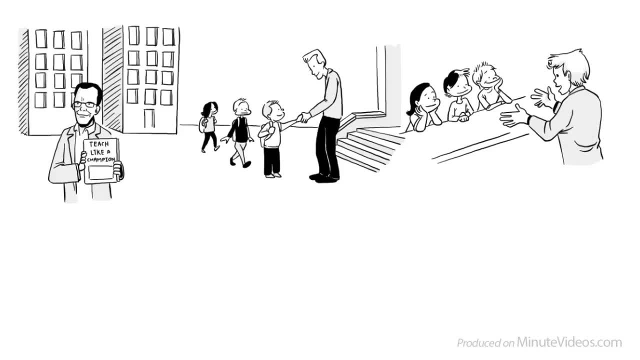 They also talk to the students and have a suitable attitude to the time. they need to be in time and be able to communicate with the students. Teachers say that these students learn well. The students are trained to be more creative and open and are even more attentive to real 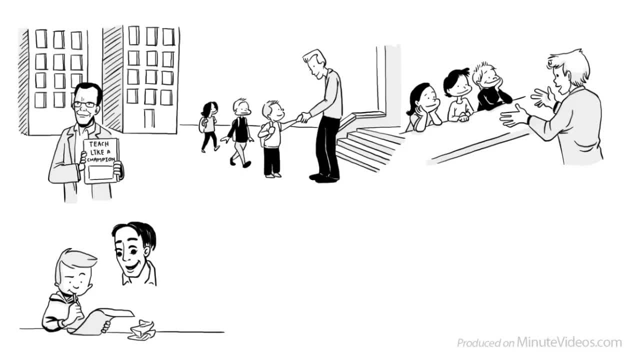 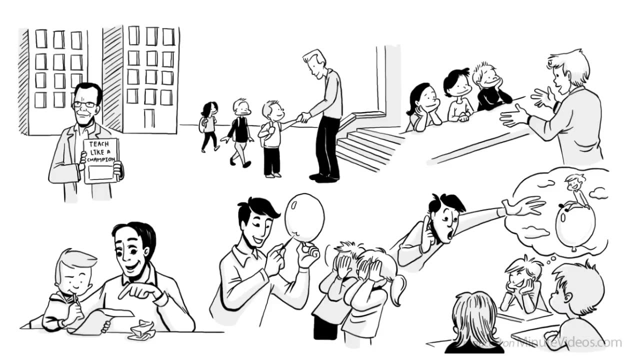 life more, But maybe most importantly, great teachers first get their students excited and then keep their attention through storytelling and engaging activities that spark their imaginations. Other examples of running a course: A paper published by Stanford Institute for Creative Learning, published on August 23,. 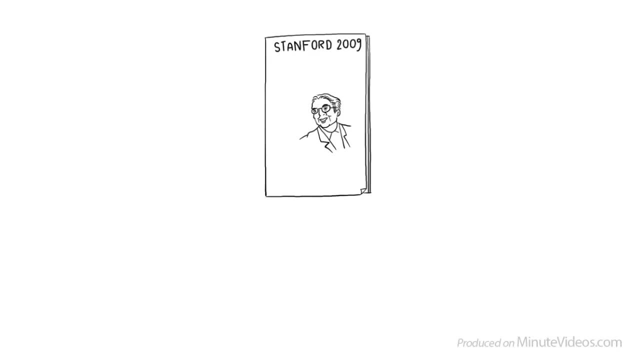 probably the second most recent paper published by the Fulbright Scholars lln was published in Adelaide, United Kingdom. 2009 showed that leadership makes a big difference too. At low-performing schools, principals hardly ever show up in the classrooms, but instead. 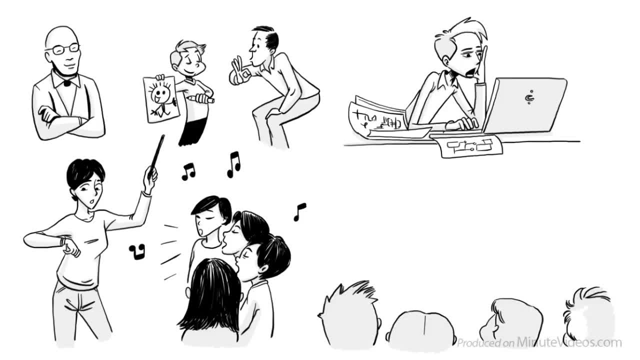 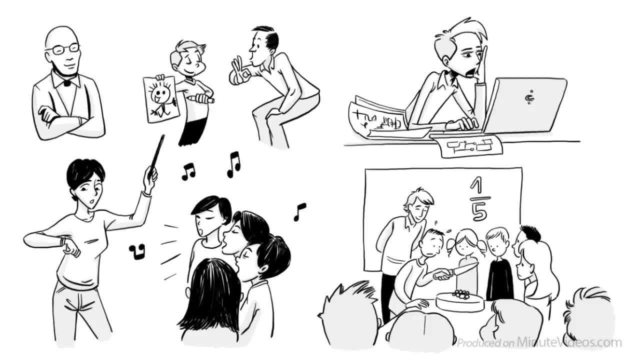 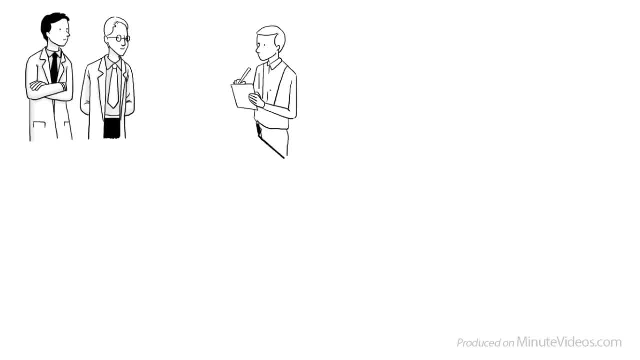 they teach their students how to learn it for themselves. In order to get it right, we have to treat and train teachers like brain surgeons. After all, they operate on human brains. Like aspiring doctors, they are best trained in the field where they receive professional feedback when they make. 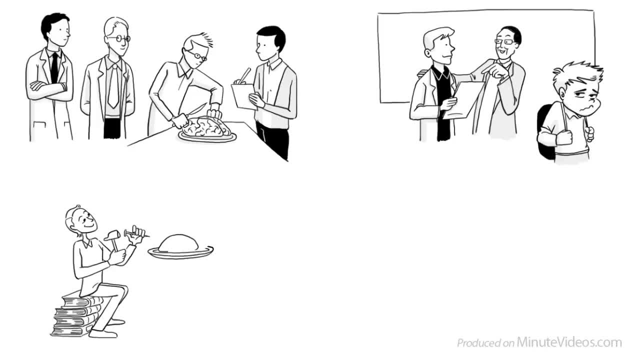 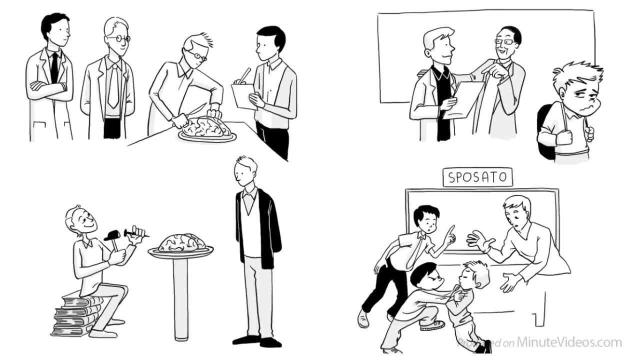 mistakes. Effective schools of education therefore train teaching like a craft rather than an abstract science. At Spasato, a graduate school of education known for creating effective teachers, students spend a lot of their time tutoring or assisting professionals. Teachers who are already in the classroom need regular professional 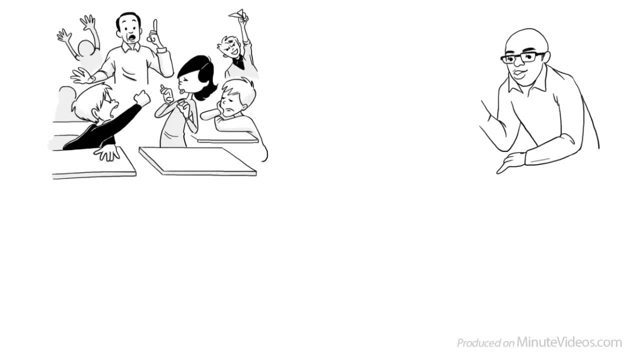 feedback on the job. A vast study by Roland Frye from Harvard found that teachers who were already in the classroom need regular professional feedback on the job, and then they don't get- And the students who are already learning there, because there's no social timing at all. 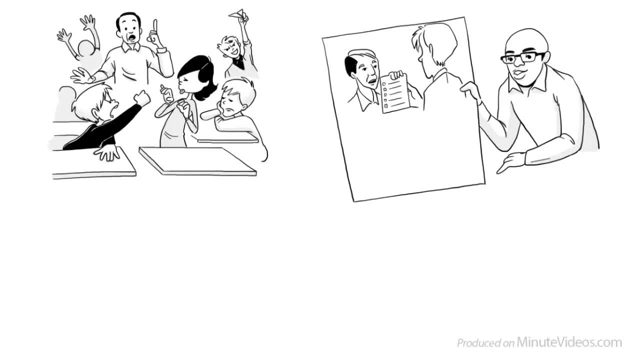 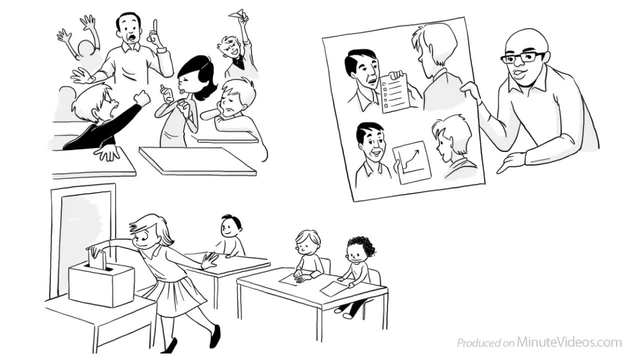 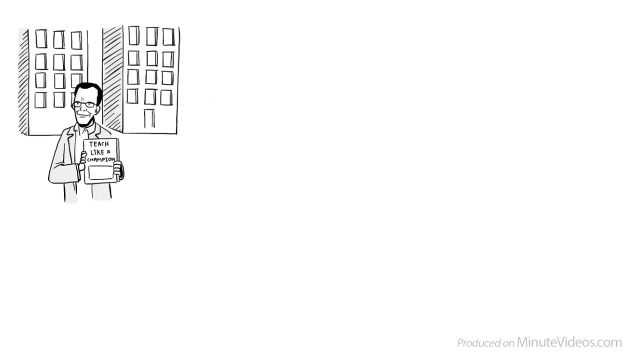 Teachers who receive precise instructions, together with specific, regular feedback from a lead teacher, will improve the most. Other good ideas to improve teachers are to ask the students for feedback or to record lessons on video and let the teachers watch themselves. Doug Lamov, founder of Uncommon Schools and author of Teach Like a Champion, identified 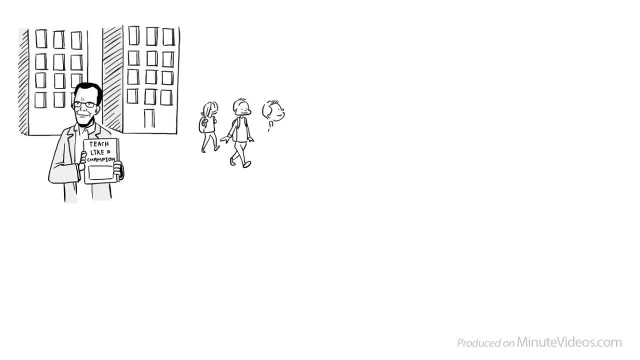 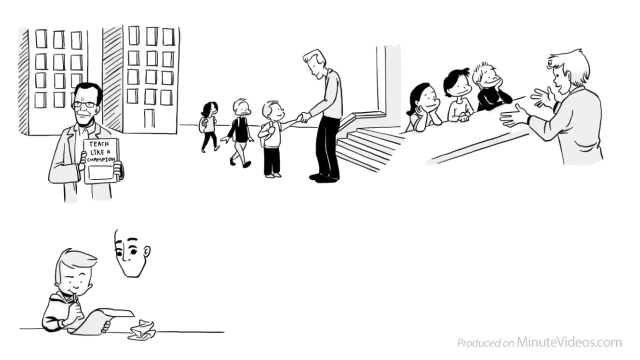 many methods that great teachers use. They greet each student at the door so students feel welcomed and acknowledged of their existence. Later they use a strong voice and don't stop talking until they have everyone's attention. Plus, they teach for mastery learning to ensure students get it 100% right before they proceed. 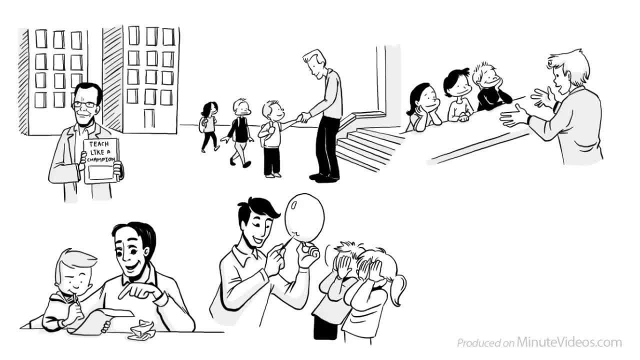 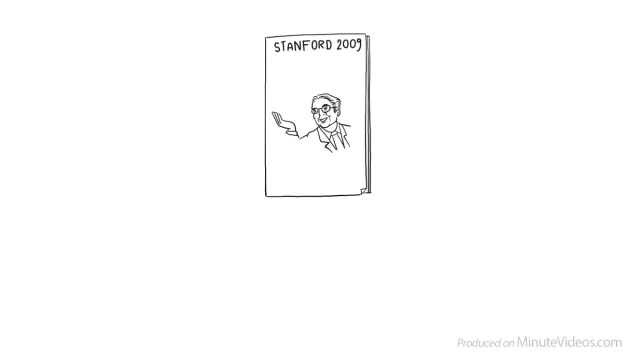 But maybe most importantly, great teachers first get their students excited and then keep their attention through storytelling and engaging activities that spark their imaginations. A paper published by Stanford in 2009 showed that leadership makes a big difference too. At low-performing schools, principals hardly ever show up in the classrooms, but instead 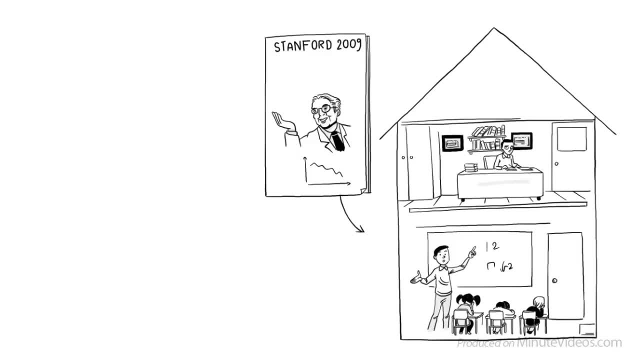 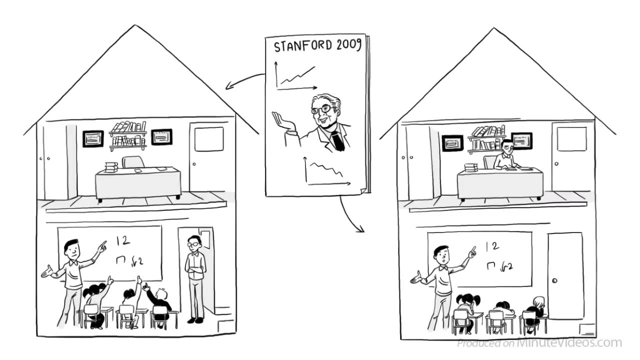 spend most of their time on administration documents or finance. Schools with better students have principals that get out of their office and spend a lot of time in the classrooms supervising and developing the teachers. Together they can make a big difference. They can make a difference in their students' life. 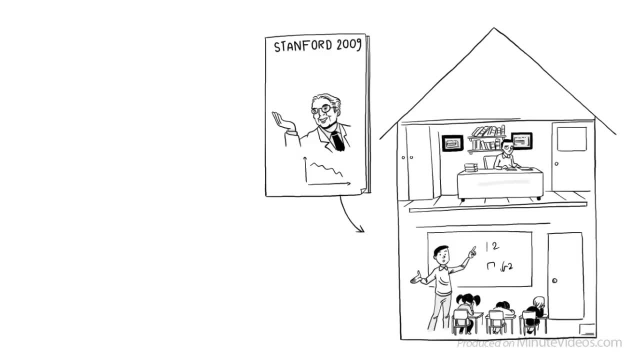 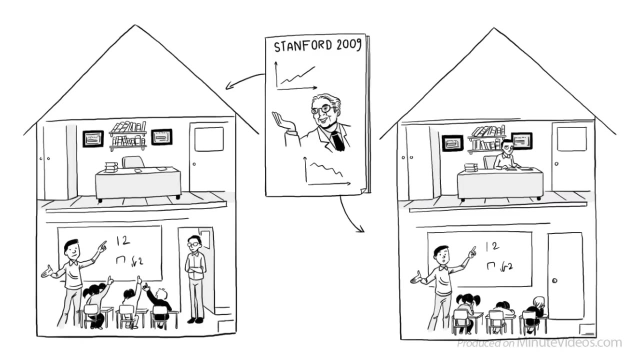 spend most of their time on administration documents or finance. Schools with better students have principals that get out of their office and spend a lot of time in the classrooms supervising and developing the teachers. Together, they can make a big difference in their students' life. 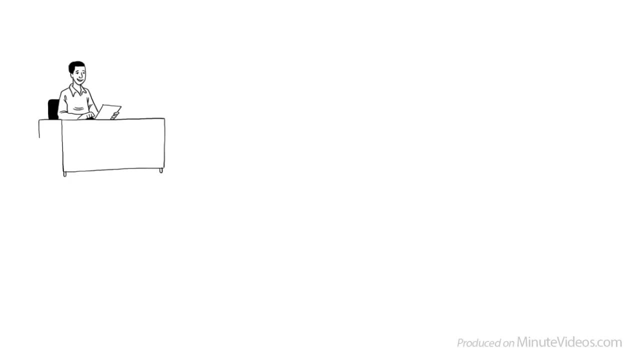 Economist Raj Chetty and his team analyzed the data of 2.5 million US students and 18 million test results. He thinks that instructors who are good at teaching to the test have a big impact. On average, having such a teacher for just one year raises the students' test scores. 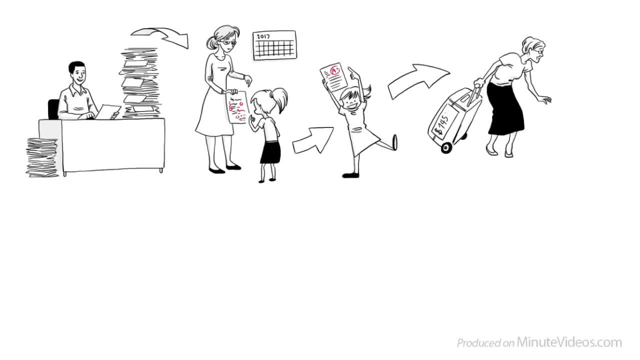 and cumulative lifetime income by 14,500 in 2019.. On early childhood education, he has another hypothesis. Great kindergarten teachers help to develop social skills, discipline and character. Their impact does not improve test scores during the school years but, surprisingly, 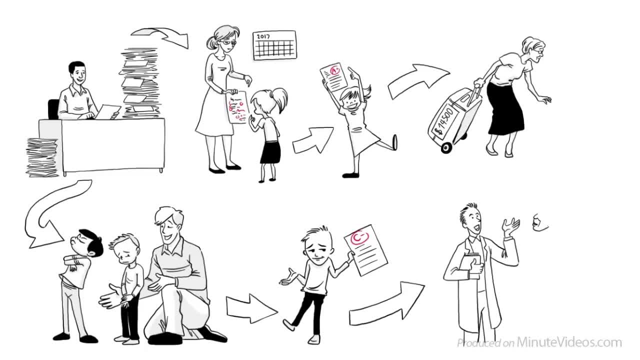 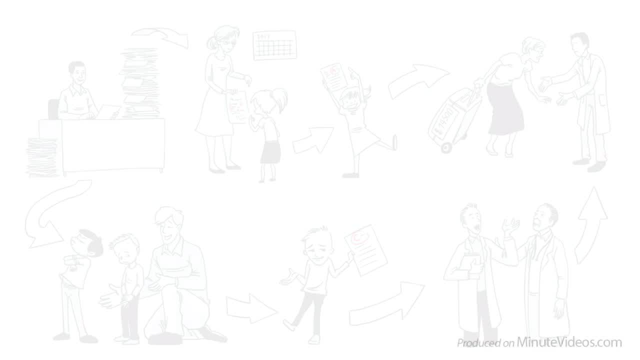 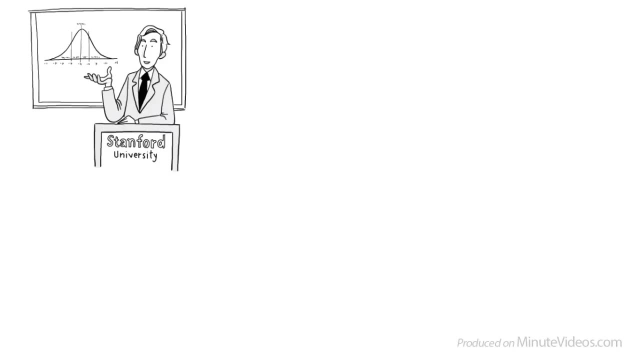 re-emerges years later when their former students apply those skills to advance in their careers and find meaningful and well-paying jobs. Eric Hanushek, Professor at Stanford University, Stanford University computed how much good teachers really matter. He found out that top teachers get students to learn 50 percent more each year than an 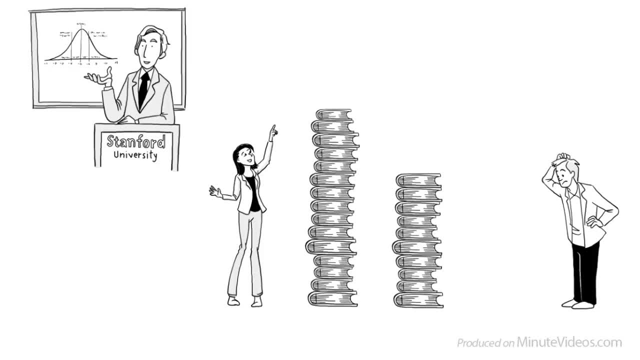 average instructor, Poorly trained ones, just half of the average. That means that 10 years at school can either result in 15 years of actual learning or just a mere five years. This is a massive difference that mainly hurts children from low-income families who can't. 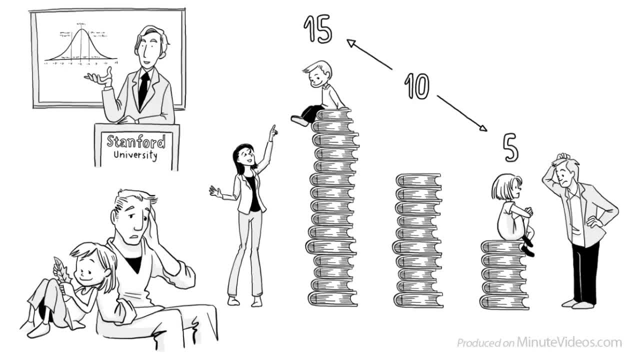 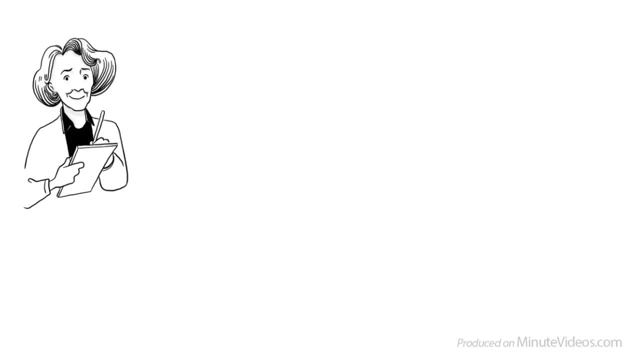 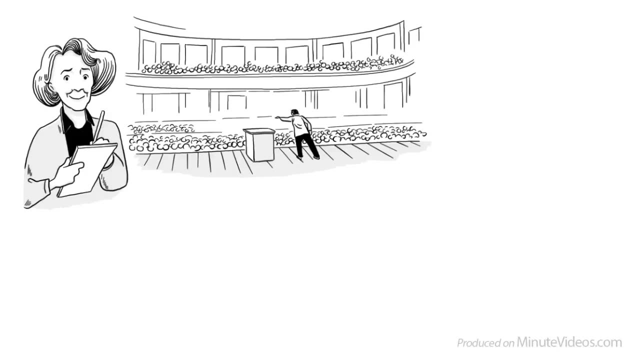 afford extra classes or school fees. American novelist Gail Godwin once wrote: Good teaching is one-fourth preparation and three-fourths pure theater. To see great actors in action, watch Michael Sandel from Harvard teach law, Robert Sapolsky from Stanford teach behavioral biology, Walter Mischel from MIT teach physics. or Mr Hester.